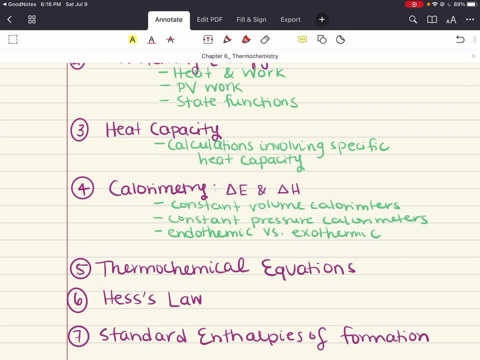 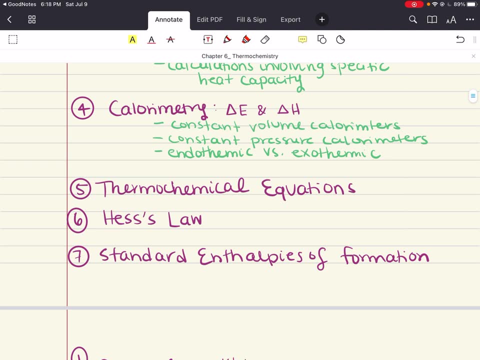 we're going to define what heat capacity is and then do calculations involving specific heat capacity. Our fourth topic is going to be calorimetry. We're going to talk about constant volume calorimetry, constant pressure calorimetry and then even define some really important. 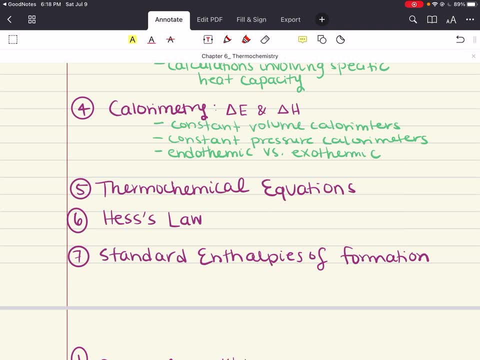 terminology, like what endothermic versus exothermic is. Fifth topic is going to be thermochemical equations. This is going to help us segue into Hess's law, which is our sixth topic, and then standard enthalpies of formation to end off this. 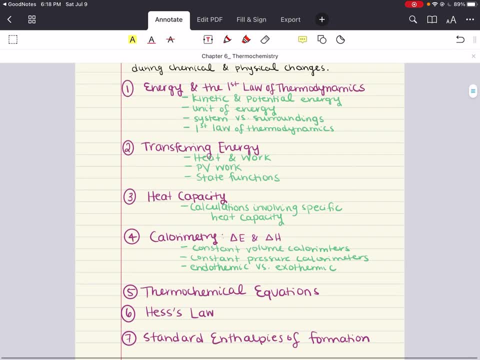 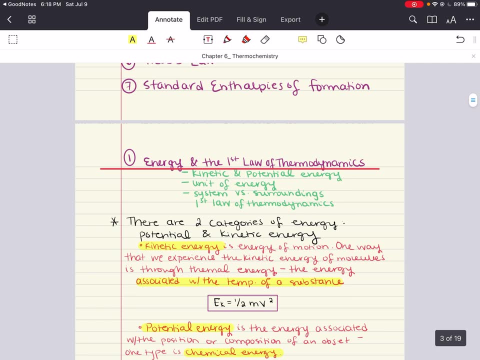 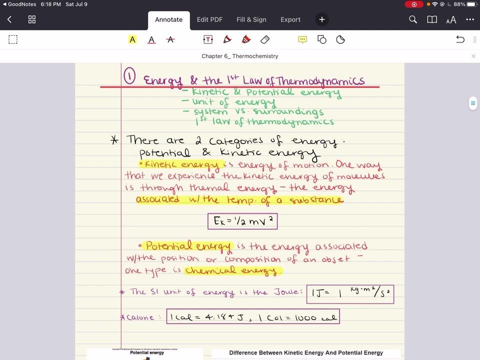 chapter. So these are the seven topics, big category topics- that we're going to cover in this chapter alone. All right, so let's go ahead and get started with energy, our first topic, energy, and the first law of thermodynamics. So important to start off by saying there are two. 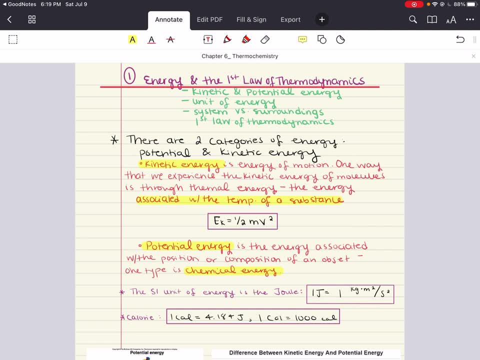 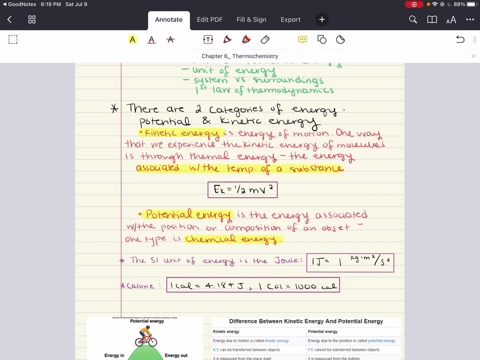 centuries of energy. We have kinetic energy and potential energy. Kinetic energy is the energy that's going to be associated with an object in motion. For example, consider a molecule in motion, a molecule moving around. All right, that molecule in motion possesses kinetic energy. Then, if it. 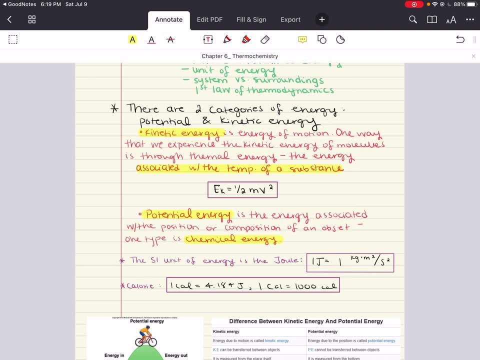 collides with another molecule, it might transfer its molecule to the other molecule it just collided with. If it collides with another molecule, it might transfer its molecule to the other molecule it just collided with. That molecule will move around, and so it has to process this obsession. 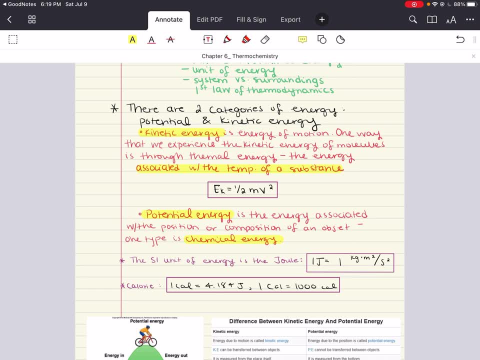 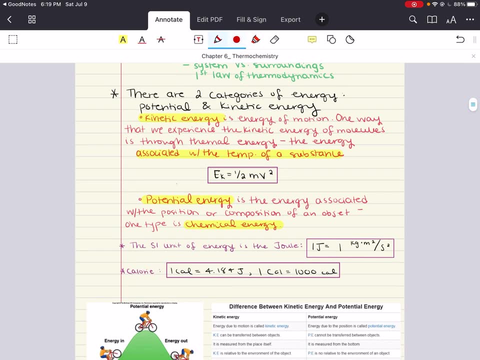 move, it now possesses kinetic energy. all right, We can figure out the kinetic energy of a molecule using the following equation: all right, One half mv squared. all right, If you've taken general chemistry, you have for sure encountered this equation. all right, One way that we experience. 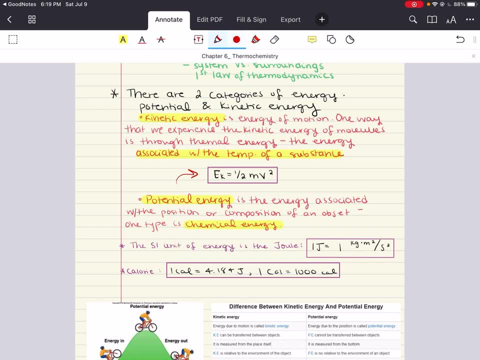 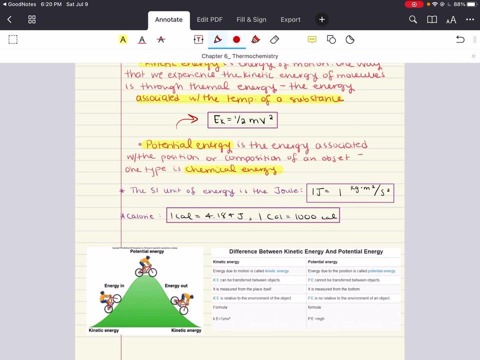 kinetic energy of molecules is, through thermal energy, the energy associated with the temperature of a substance. all right Now the second category of energy is potential energy. Potential energy can be thought of as stored energy or, more precisely, energy associated with the position or 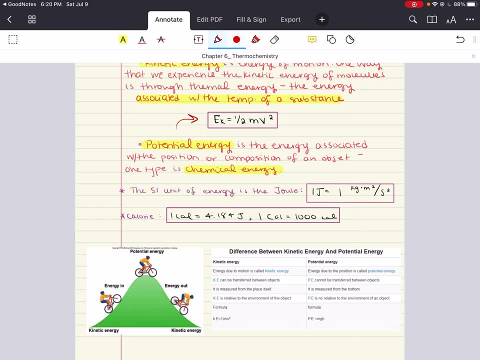 composition of an object. So, for example, holding an object five feet above the ground, right, You're standing still. you have an object that you hold in both hands, all right, And it's about, say, five, six feet above ground, That object sitting in your hand, not moving. 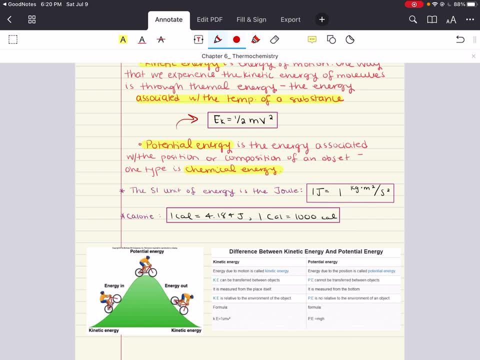 possesses potential energy due to its position in the gravitational field. all right, Then when you drop it, that potential energy converts to kinetic energy as it falls, as it moves down from your hands all the way to the floor. all right, So that's how you kind of want to think. 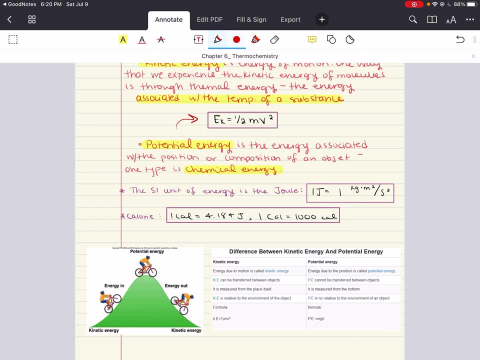 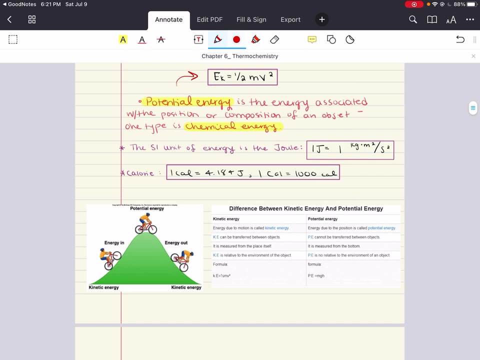 about potential energy versus kinetic energy. Now, one type of potential energy, all right, is chemical energy. So an example of something that has chemical energy: battery. A battery possesses chemical energy resulting from the relative positions of electrons and nuclei of the atoms and molecules in the battery. Now, when a chemical reaction occurs, 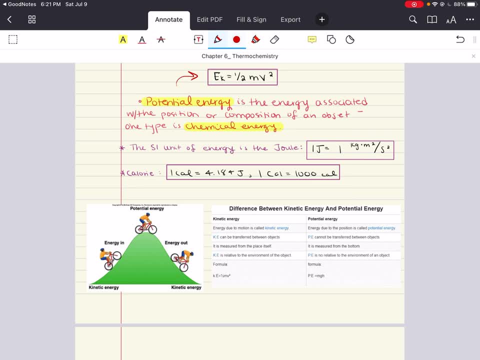 electrons and nuclei. they're going to change their position so that energy is absorbed or released. all right, And that's kind of like a little snippet of how batteries work. We'll be getting into that soon. all right, Now an important thing to remember when 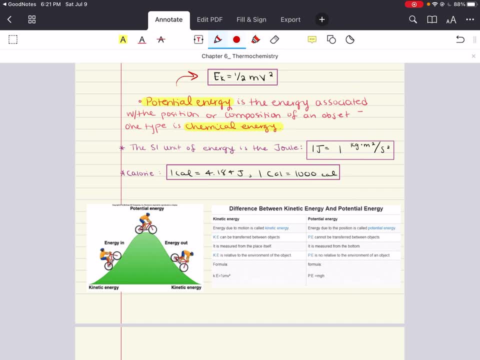 discussing energy, is the unit of energy right? Stating out a value without a unit is always pointless, especially if you're really trying to talk about energy. have to slap on appropriate units when talking about energy. all right, Now the unit of energy that we're going to be talking. 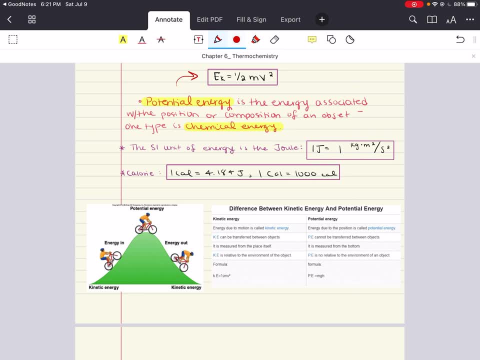 and using is and is the unit of energy, I'm sorry, is a joule, And a joule is defined as you see right here. One joule is one kilogram times meter squared over six Seconds squared. all right, Now you should also be familiar with the more English unit for: 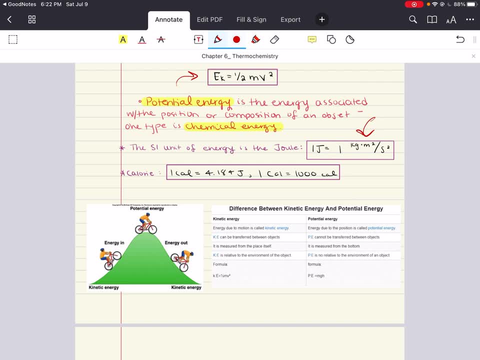 energy. That's the calorie. all right, The calorie is the amount of heat required to raise the temperature of one gram of water by one degree Celsius. The relationship between joule and calorie, all right, is this: One calorie equals 4.184 joule. Now, this is different Calorie with. 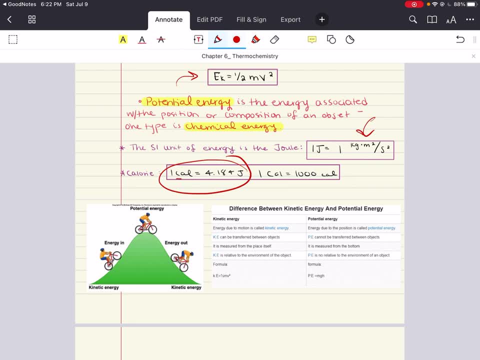 a lowercase C is different than the calorie with an uppercase C. all right. The uppercase calorie is that familiar nutritional term that you've encountered, And it's actually equivalent to 1,000 lowercase calories. all right, So keep that in mind Now in thermodynamics, all right, whenever we want. 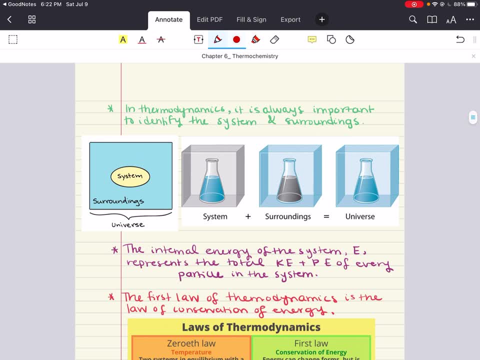 to talk about thermodynamics, it's important to be able to distinguish between the system and the surroundings. all right, The system is the part of the universe that we single out for the study. The surroundings include everything else in the universe. Now, this system plus the surroundings equals the. 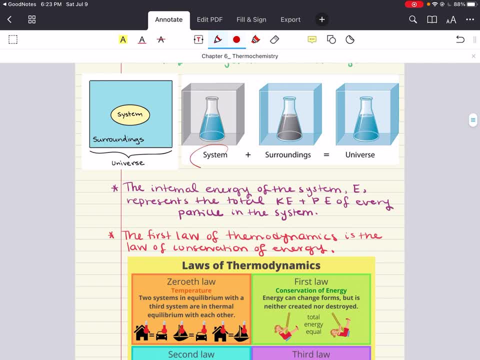 universe. That's kind of how we like to think about it, That system plus surroundings, equal universe. Now when we say this, we can generalize the universe, all right, We can generalize the universe because that's a lot. We can generalize the universe because that's a lot, And we can 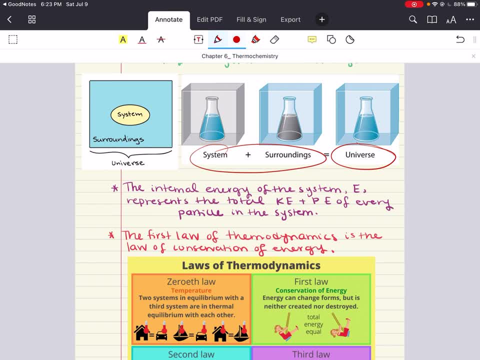 to talk about. We can generalize the universe to the rest of the immediate surrounding in an experiment or observation. In this chapter and mostly in general chemistry, the system will always include the molecules and atoms that are undergoing chemical change. So the choice of 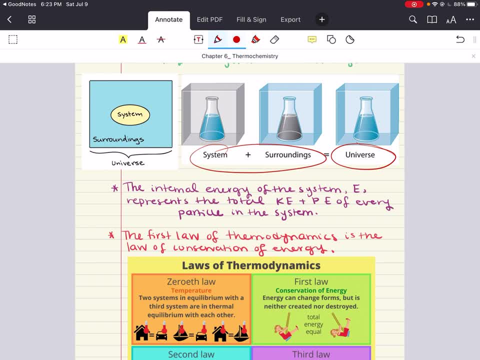 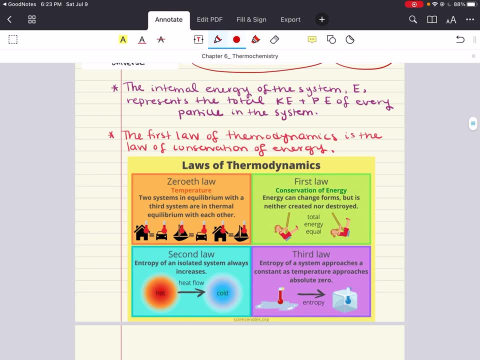 system will usually be pretty obvious. Now, having selected an appropriate system, our next step is to describe the internal energy of that system. The internal energy of the system represents the kinetic and the potential energy of every particle in the system. okay, Now that. 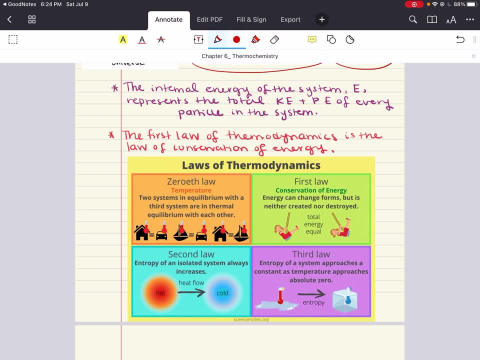 sounds kind of crazy. You have to know all this information, kinetic and potential energy all right of every particle in the system. Even for simple systems, this would be practically unachievable. all right, So, even though we might not always know the exact internal 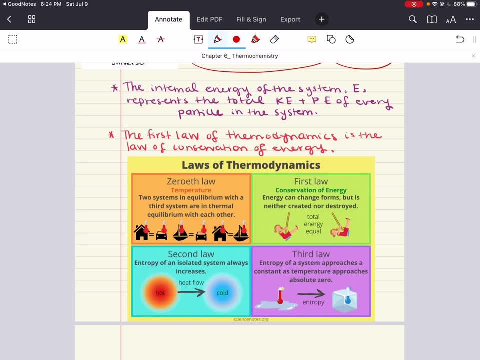 energy of every particle in the system. we have to know all this information all right, Because it seems kind of impractical to know all the kinetic and potential energy of every particle. we can actually usually determine how much a system changes its internal energy And 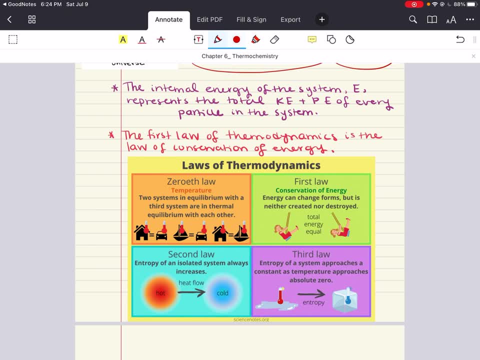 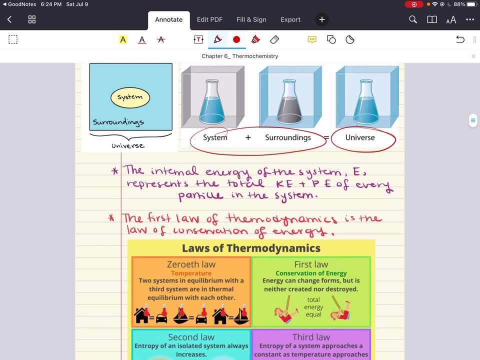 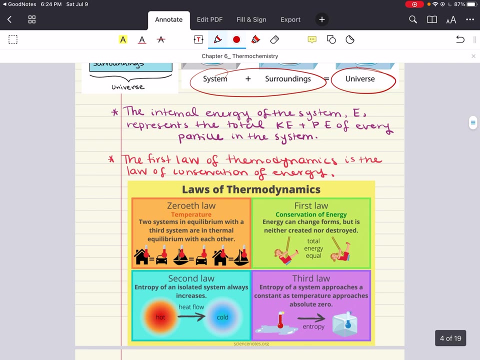 therefore, we begin to talk about energy in terms of change of energy, or delta E. Delta E represents the change in internal energy. all right, So you can think about it as final minus initial, All right. so now, keeping that in mind, all right, and knowing that this delta E, this change in, 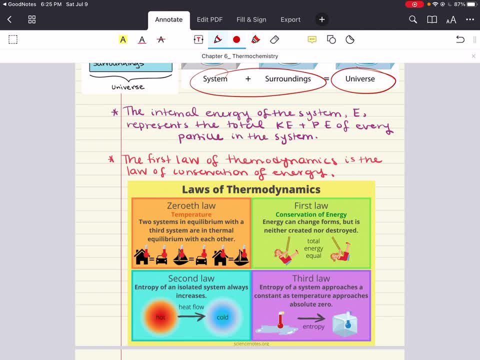 energy is going to tell us the direction of energy flow. all right, How is it going to do with that? Well, if delta E is negative, then the system loses energy, And if delta E is positive, then the system gains energy. And that makes sense, if you try to think of yourself like 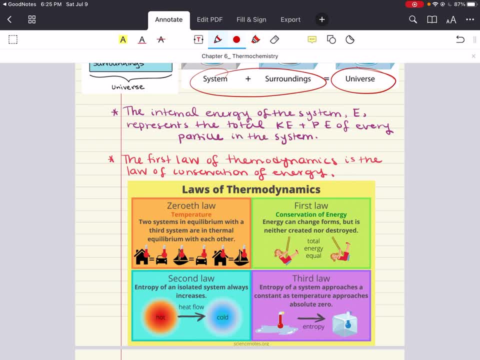 close your eyes, pretend you're the system. all right. If you expel energy, all right. you're going to have a negative delta E right Because you're getting rid of that energy, all right. But if you gain some energy, then your delta E right. 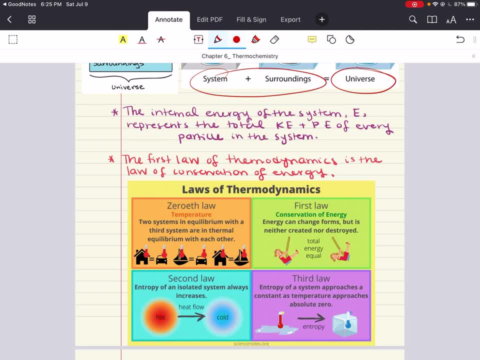 your internal energy is going to be positive. all right. With all that in mind, now we can finally discuss the first law of thermodynamics. This first law of thermodynamics is also known as the law of conservation of energy. It states that, although energy can be converted from, 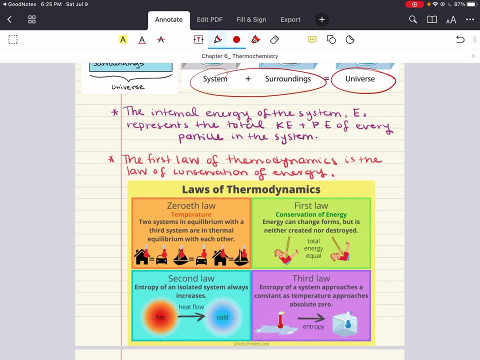 water to water. it can also be converted from water to water to water, And so if you convert from one form to another, it cannot be created or destroyed. So what that means is the total energy of the universe is going to remain constant. all right, It's going to remain. 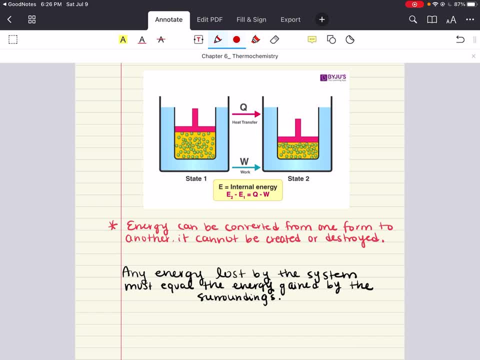 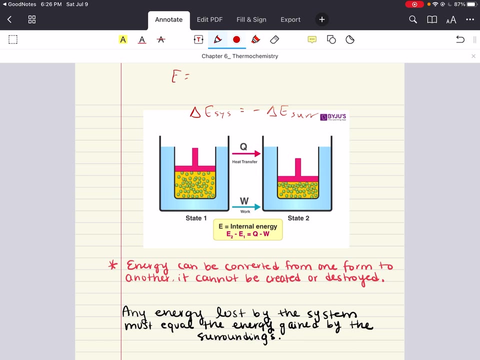 constant. So delta E of the system all right is going to equal to the minus delta E of the surroundings all right. That's a consequence of saying that if all energy stays the same, all right. energy is not created or destroyed, it's just converted from one form or another. 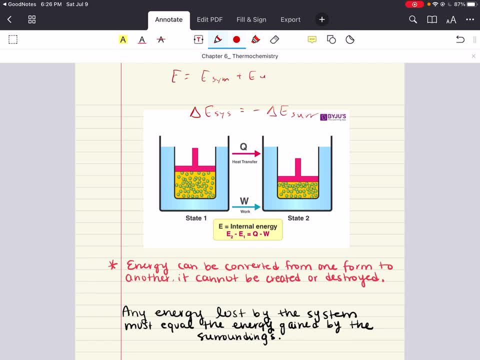 then the energy of the system plus energy of the surroundings is going to equal the energy of the universe. all right, So, similarly, the total energy of the universe is constant. Any energy lost by the system must be gained by the surrounding, and vice versa, all right. 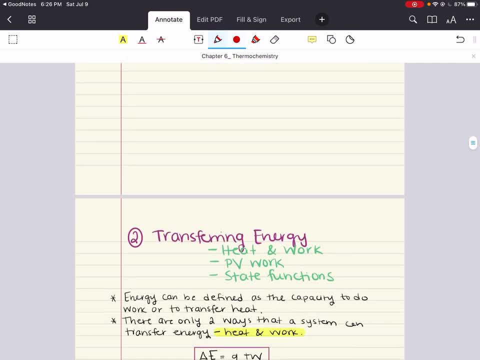 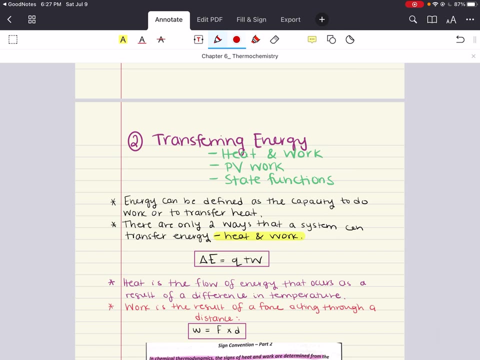 Fantastic, Fantastic. Now that we have covered that, that's all kind of like preliminary background information, we can move on to discussing how energy can even be transferred to begin with. all right, And so with that, it is time for us to give energy a formal and proper definition. 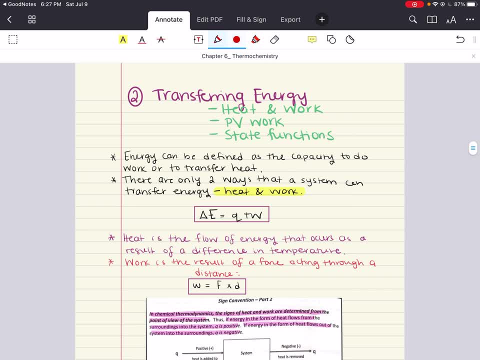 all right. Energy is going to be defined as the capacity to do work or transfer heat. The capacity to do work or transfer heat. That means we can write a formula for energy where energy all right- is defined as the capacity to do work. 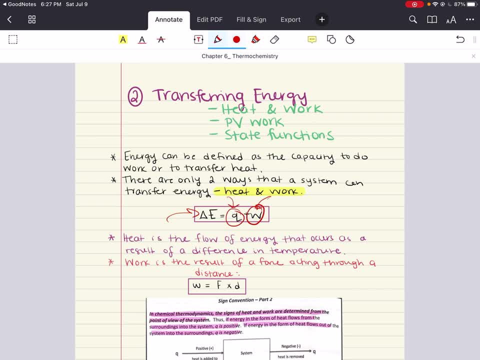 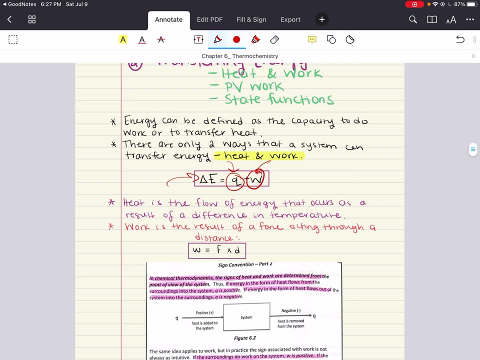 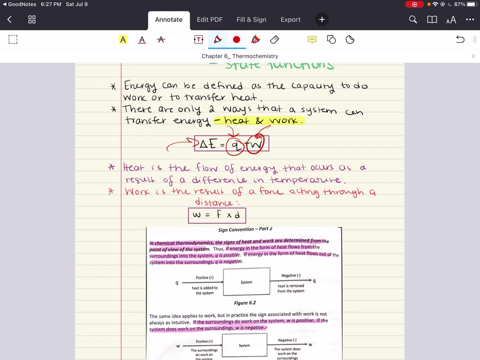 which is what this W term is, or transfer heat, which is what this Q term is. all right, Now we have to go ahead and define what those two things are. What's heat? What's work? Heat is the flow of energy that occurs as a result of a difference in temperature. When energy is, 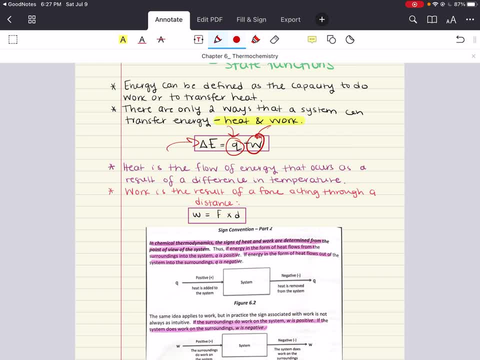 transformed as heat. the direction of heat is transformed as heat. When heat is transformed as energy, the direction of energy transfer is going to always be from hotter object to colder object. One thing to notice is that heat is not the same as temperature. Heat is not the same as. 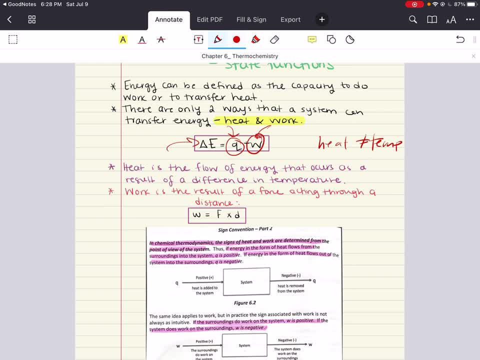 temperature. all right, Temperature is the measure of kinetic energy of a system. Heat is the measure of transfer of kinetic energy from one system to another. Now another thing: heat is not energy. Heat is one of two ways that energy can be transferred, And I 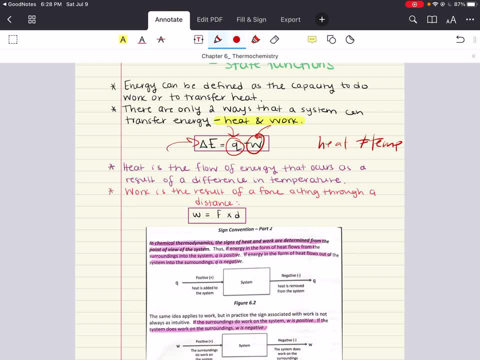 know that's kind of weird. all right, I understand that's a weird concept, especially if you're hearing it for the first time. all right, But that's okay, Just remember: heat is one way that energy can be transferred. It's not energy, though, all right. Now the second thing. 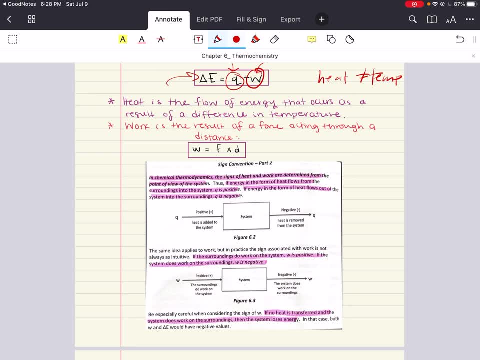 the second way that energy can be transferred, like we said, is work. Work is the result of a force acting through a difference, So we can actually write a formula for work. Work is the force acting through a distance. Force times distance equals. 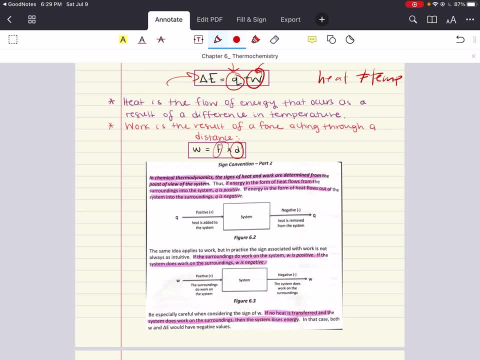 work. Now, in chemical thermodynamics, the sign of heat and work are determined from the point of view of the system. So here's your system, all right. If you add heat to the system, all right, All right, your heat is going to be positive valued If heat is removed from the system. 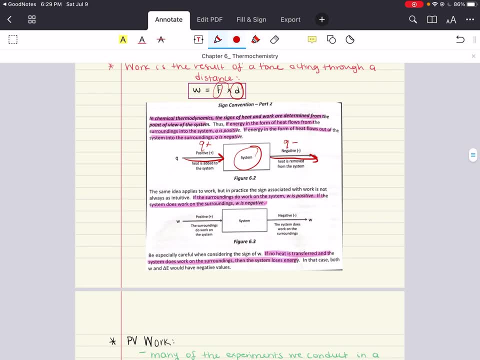 heat gets a negative value. all right, Now system: if the surroundings does work on the system, all right. work has a positive value. If the system does work on the surroundings, work has a negative value. So I really like these two diagrams. 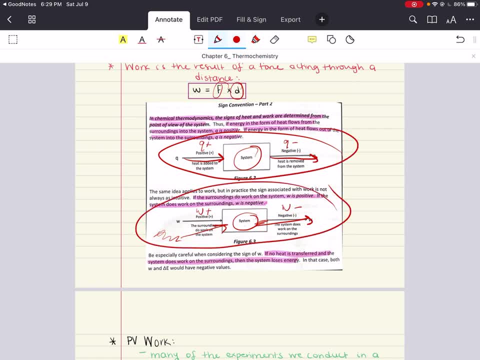 to help you remember how to assign signs to work and heat values so that when you're asked a question like determine the change of internal energy in a system, you can assign the proper signs to the heat and the work values that you're given so you can calculate internal energy for a system. 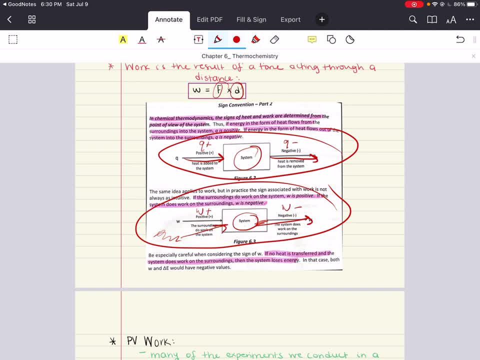 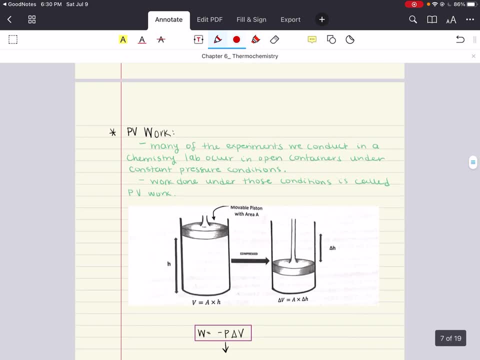 properly, all right, And we're going to get to doing problems like that in just a second. We want cover. one more thing here, all right, and that's pressure volume work. Now, many of the experiments we conduct in our chemistry lab course, for example, they're going to occur in open containers. 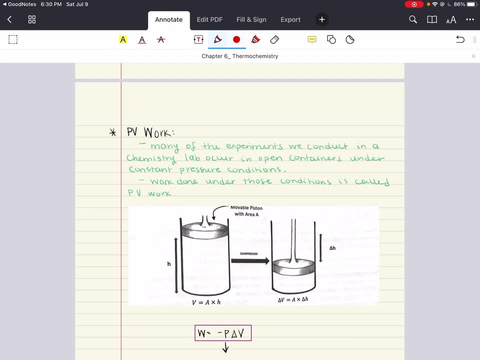 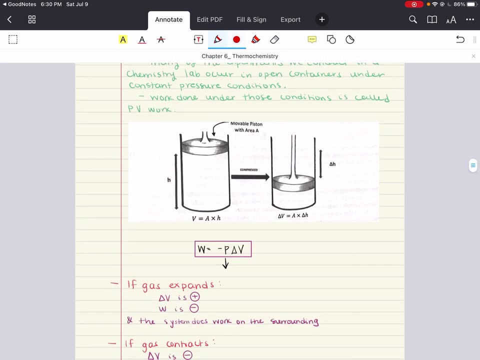 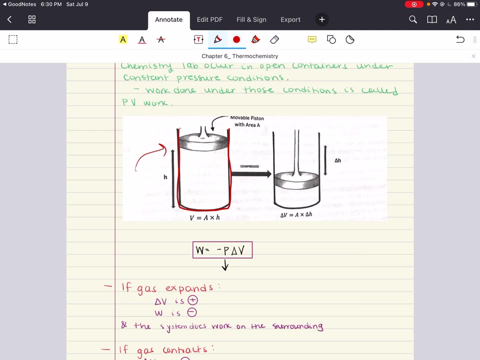 under constant pressure conditions. This is going to be called pressure volume work. all right, Let's take all right this as an example. We have this movable piston inside a beaker. all right, movable piston, cool. all right. Now by exerting a force on the piston. 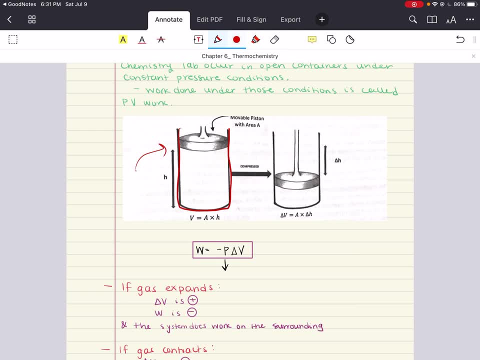 okay, by exerting a force on the piston, we can move the piston by a distance of delta h. all right, we can move it by a distance of delta h. If we bring it down, then the change here in distance is delta h. all right, Since work is defined as the force of the piston. 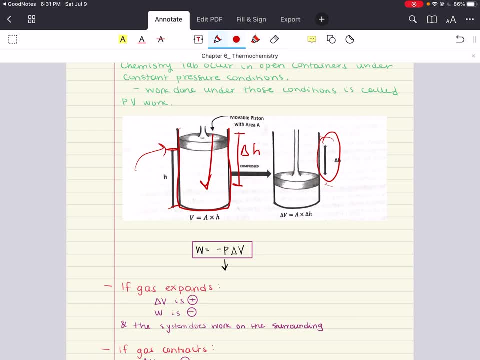 applied over the distance, then that means when we compress the surroundings, all right, we're doing work on the system. all right, Surroundings is doing work on the system, because this is the system. here's the piston: we force it down where the surroundings is doing work. 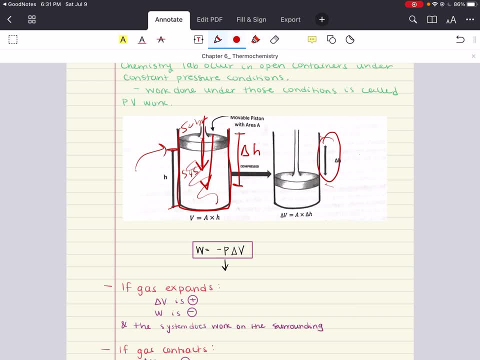 on the system. What does that mean? That means the sign of work will be positive. all right, Awesome. Now the point here. the point is that through some calculations, we're going to get an expression for work that is: work equals minus p, delta, v. all right, Through some mathematical workup. 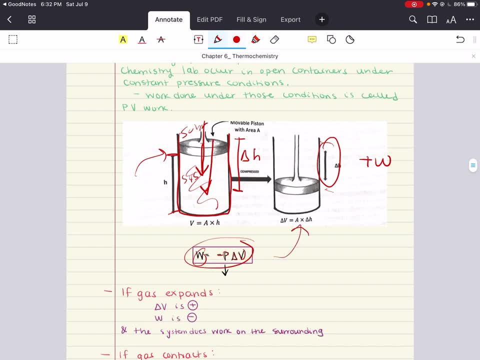 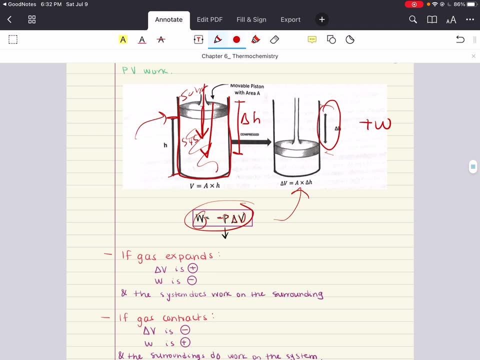 we're going to get this expression to describe the work that we have done by moving a piston. all right, And I'm not going to go over the math right here, but I can definitely post it. if you're interested in the proof, I'm happy to do that. But the point again is that through some 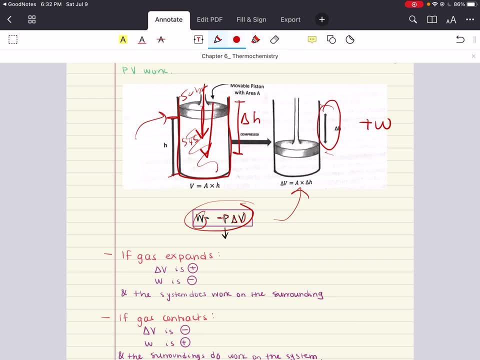 calculation, we're going to get an expression for work. all right, that is, work equals negative pressure, change of volume. all right, So we can describe work through this change in volume that we've done by moving the piston and, as a consequence, the change of pressure that occurs. 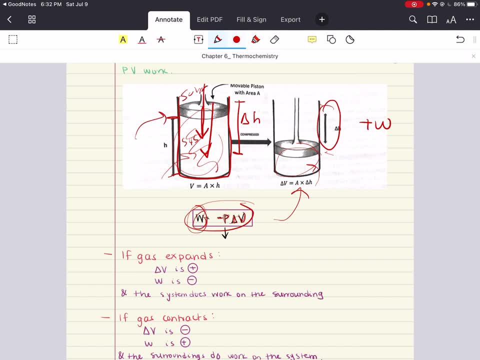 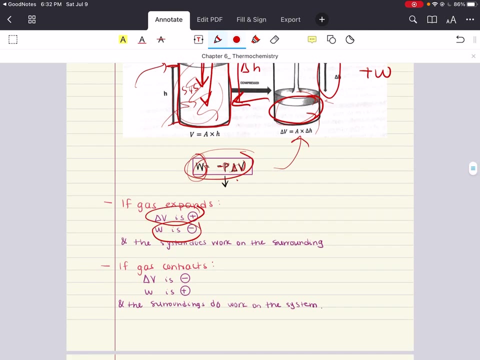 inside this, all right, That makes sense. What this means is if the gas expands, if you're going from small volume to large volume, the gas expands. then delta v is positive, all right, and work is negative. That means that the system does work on the surroundings, The system. 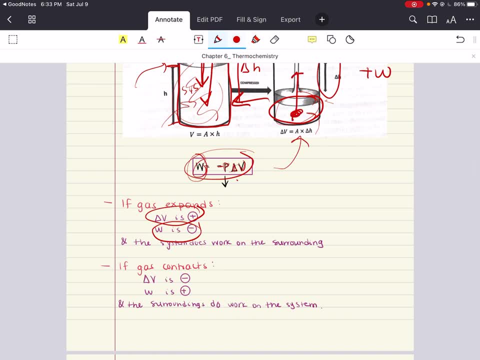 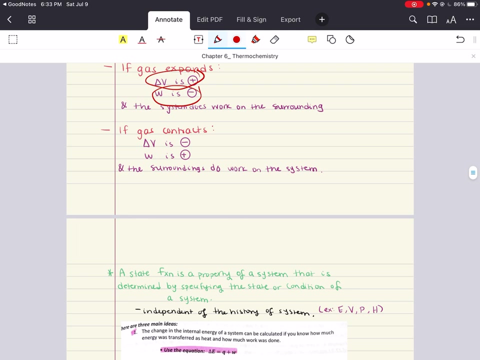 all right. does work to push the piston up? all right, Expand the volume. work is negative. If the gas contracts, then delta v is negative. You made your volume smaller by pushing that piston in, but work is positive. The surrounding has done the work on the system all right. So that's important to know. 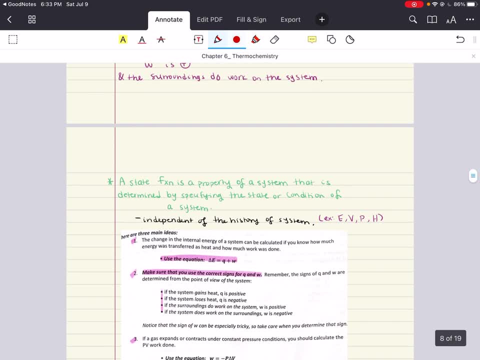 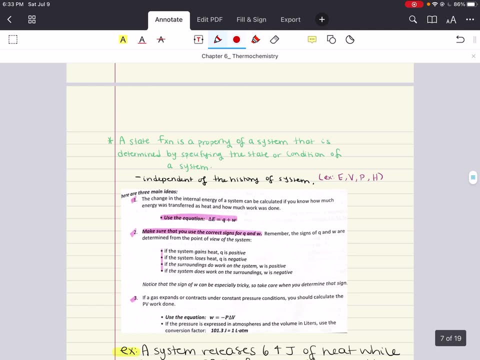 all right. Also, one more thing. that's just. I'm learning how to choose the right audio apps for you. Oops, sorry, Which one do you want to use to listen to this? Oops, don't do that, Sorry. that was my Apple Watch talking to me while I'm trying to record the video. Sorry, we're going to. 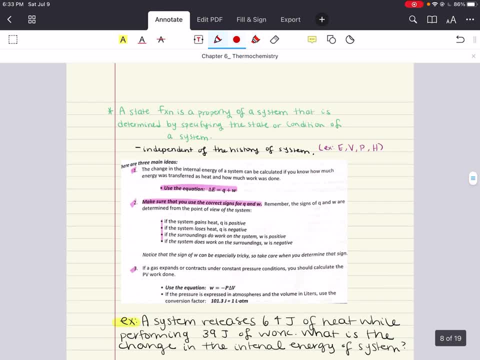 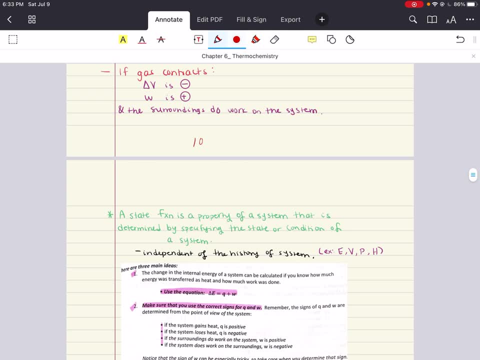 just move that, move along. all right. One quick conversion. I want to state here that might be really important when we do some practice Problems in regard to this, and that you should know. all right is that 101.3 joules equals one. 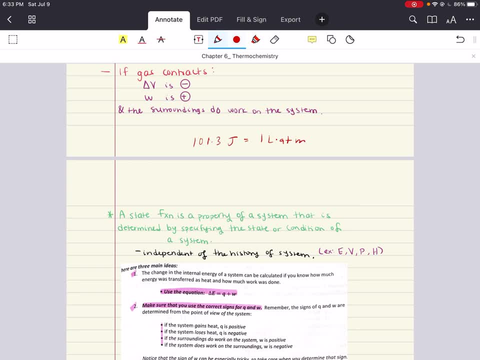 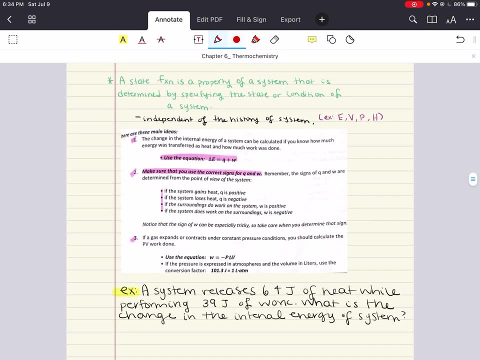 liter times, atmosphere. okay, That's something we want to keep in mind, that we might encounter and need for future problems. all right, So I just wanted to state that here. Now one more topic we want to cover before we do some examples. all right is kind of like a concept, a definition. 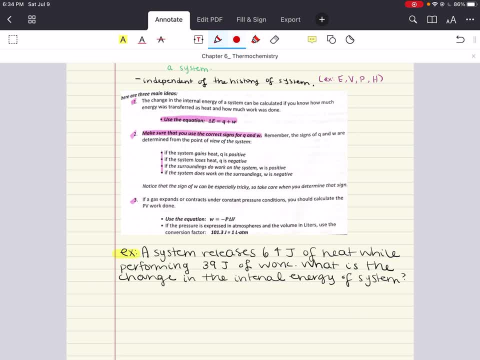 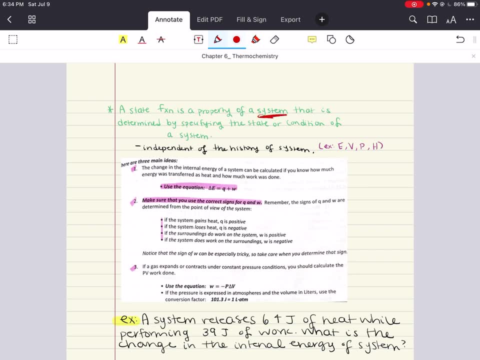 is. we want to talk about state functions. A state function is a property of a system that is determined by specifying the state or condition of a system. A state function is a property of a system, all right. that says the following: It is determined by specifying the 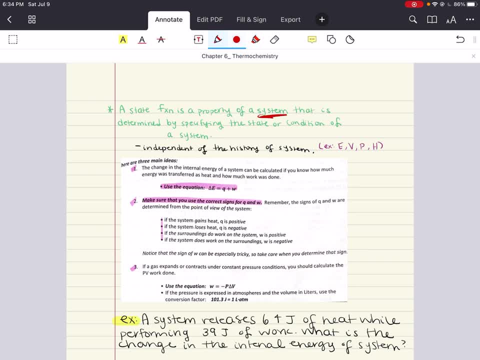 state or condition of a system. In other words, a state function is independent of the history of the system. And examples of state functions are temperature, temperature, temperature, temperature, pressure, volume, energy, enthalpy. These are all examples of state functions, all right. 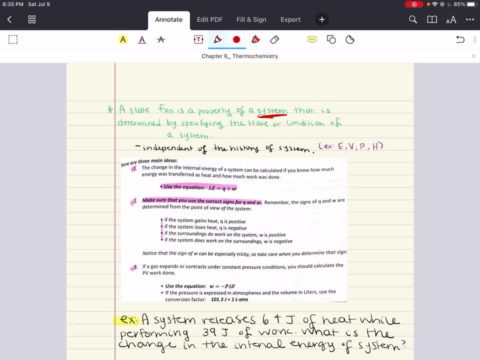 because their value is independent of the history of the system. all right, Things that are not state functions are heat and work. These values are path dependent. all right. Now we actually want to get to some practice problems, all right, And in order to do these practice, 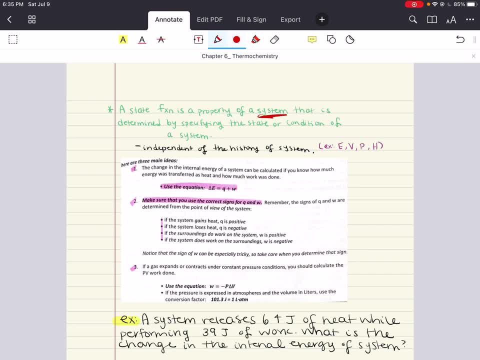 problems. there's three main ideas I want you to keep in mind. all right, The change in internal energy of a system. this is kind of a summary of what we just covered. The change in the internal energy of a system can be calculated if you know how much energy was transferred as heat. 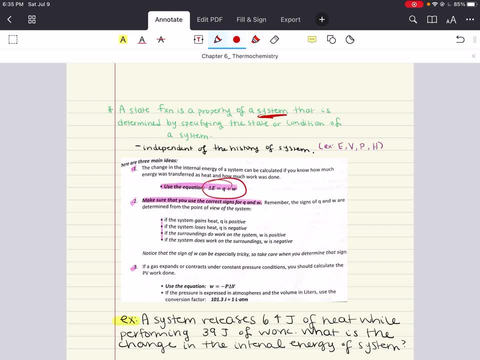 and how much work was done and we get this equation. all right, Make sure you use the correct signs for Q and W. all right, We covered this. If the system gains heat, Q is positive. If system loses heat, Q is negative. 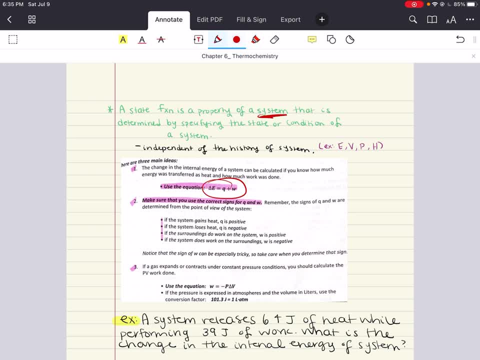 If the surroundings do work on the system, W is positive, work is positive. If the system does work on the surroundings, work is negative. all right, And last but not least, if a gas expands or contracts under constant pressure conditions, you should calculate the pressure volume work done. 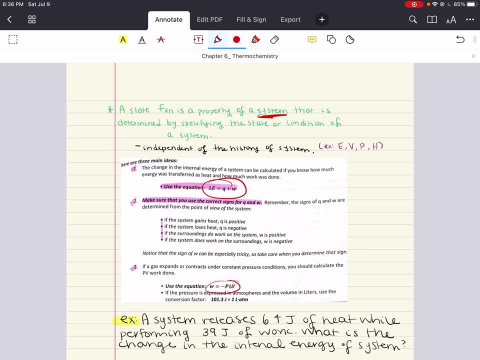 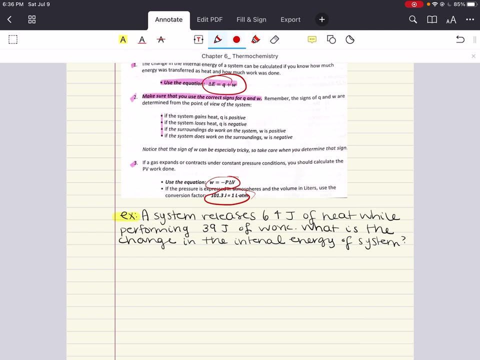 using this equation. all right, and keep in mind this conversion. all right, That's a summary of everything we just covered so far. all right, Let's do a problem. This problem says a system releases 64 joules of heat. all right, Let's. 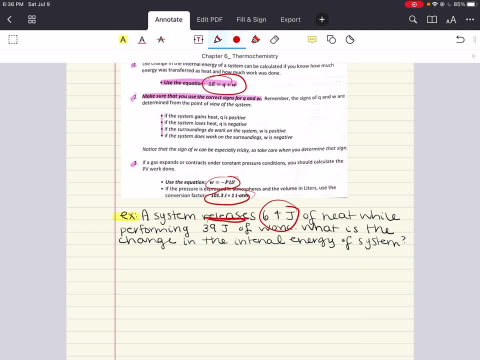 highlight this word: releases 64 joules of heat while performing. all right, while performing 39 joules of work. What is the change in the internal energy of the system? all right, We want to find the change of internal energy. We know what formula to use: Delta E equals Q plus. 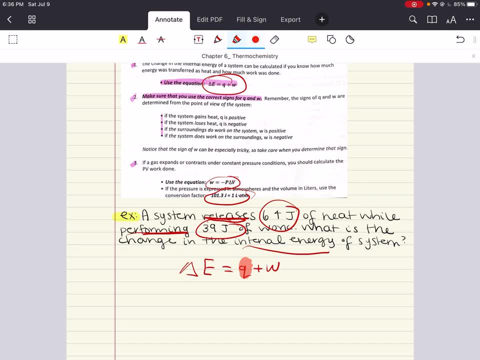 W. Guess what. They give us both values. They give us heat: It's 64 joules. They give us work: It's 39 joules. Now, the only thing we need to determine is the signs of those values. all right, So let's. 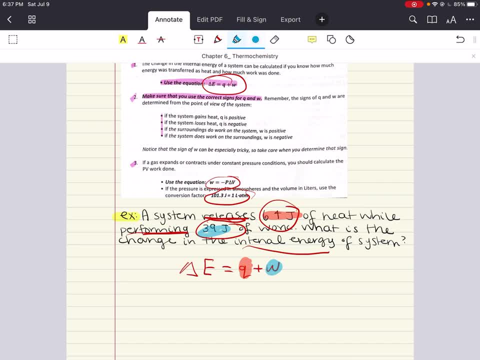 go back to the problem. It says: the system releases 64 joules of heat. So you're the system: You release 64 joules of heat. You're losing that 64 joules of heat. Therefore, heat has a negative value because you are releasing heat. 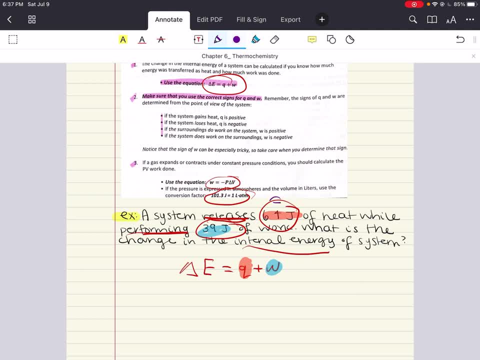 All right. So 64 joules gets a negative value. all right, It's a negative 64 joules- Fantastic. What about work? Well, remember, whenever the system does work on the surroundings, work is negative. And here, work is negative because we're saying a system performs 39 joules. 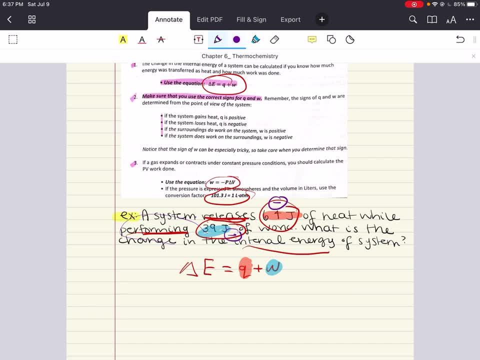 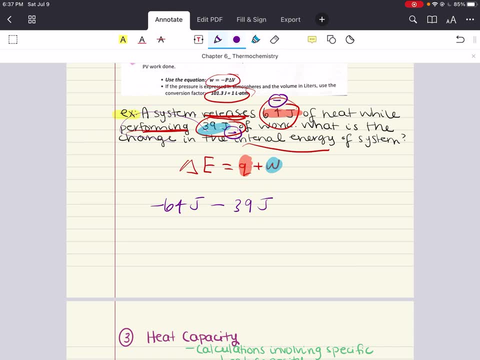 of work. So work is also negative. Both are heat And our work are negative values. all right, So, keeping that in mind, we just plug it back in the equation, put it in our calculator and what we get is minus 103 joules The change in internal 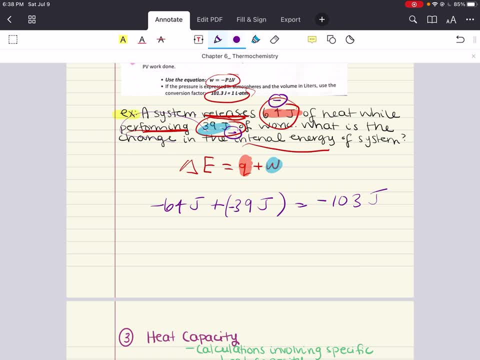 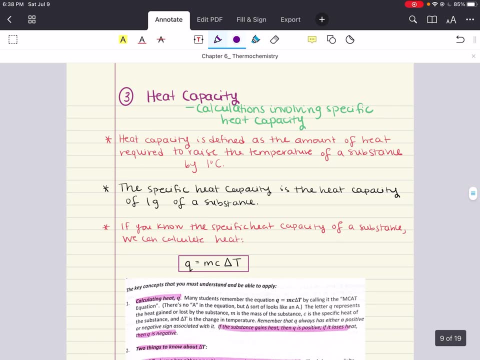 energy of a system is minus 103 joules- Fantastic, All right. Now we want to cover heat capacity. Now, although heat and temperature they're not the same, we can use changes in temperatures to calculate heat And the quantity. 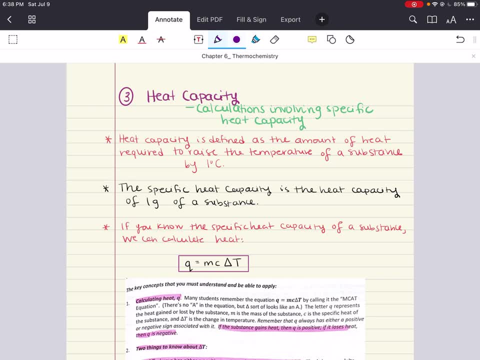 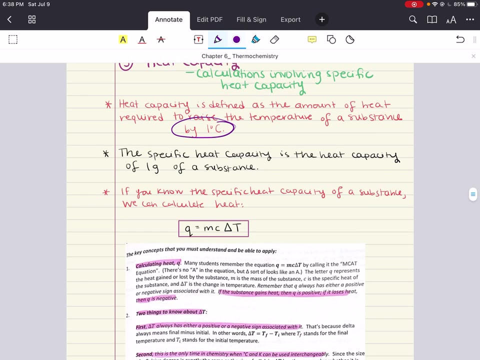 that's going to tie the two is heat capacity. Heat capacity is defined as the amount of heat required to raise the temperature of a substance by one degrees Celsius. All right, Now the specific heat capacity- all right- is the heat capacity of one gram. 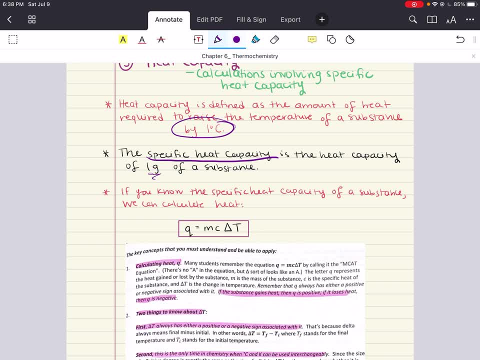 And then the molar heat capacity. all right, just to make sure you understand your terms here whenever you see them, the molar heat capacity is the amount of heat required to raise the temperature of one mole of substance by one degree. All right, Now if we know the heat. 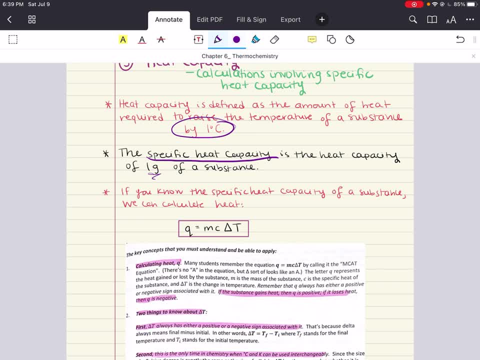 capacity of a substance. we can calculate heat, all right, using this formula: All right, Q is heat. Q equals M times C times delta T. All right, Where C is the specific heat capacity. All right, Delta T is the change in temperature, where temperature can either be in Celsius or Kelvin. 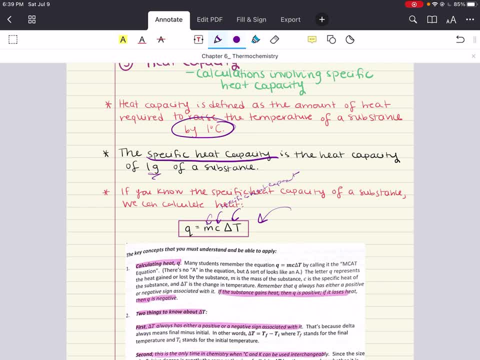 It doesn't matter, because we're talking about difference in temperature, All right. And M is your concentration? I mean, I'm sorry, M is your mass? Oh my God, M is your mass, All right. So the key concepts we have. 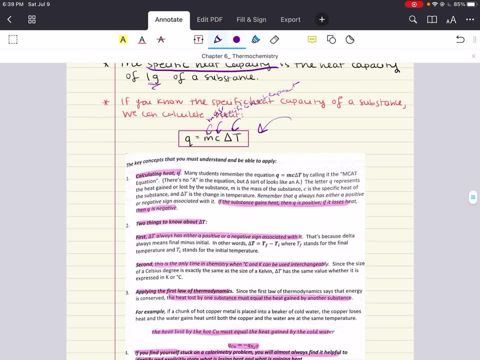 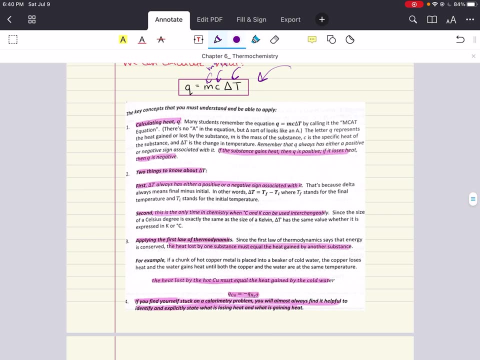 to understand, to be able to apply this. All right, We're calculating heat, That's Q. All right, If the substance gains heat, then Q is positive, And if it loses heat it's negative. All right, Two things to know about delta T, All right. Delta T always has either a positive or negative sign associated. 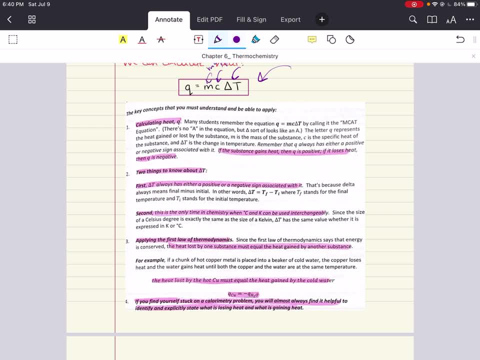 with it, All right, And it's the only time delta T is positive. All right, And it's the only time in chemistry when Celsius and Kelvin can be used interchangeably. So if you have a problem that you're trying to solve, All right, You're given a problem set and the temperature for this specific. 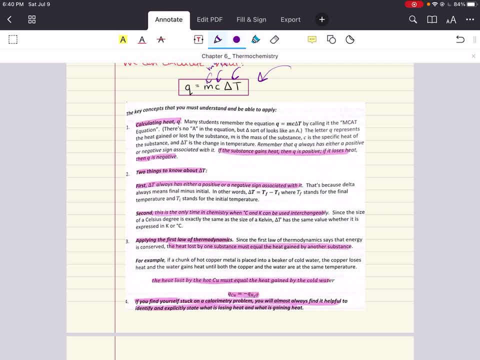 heat problem is given in Celsius, You don't need to convert it to Kelvin to do this problem, and vice versa. All right, Now applying the first law of thermodynamics, keep in mind, All right, That energy is conserved. That means the heat lost by one substance. 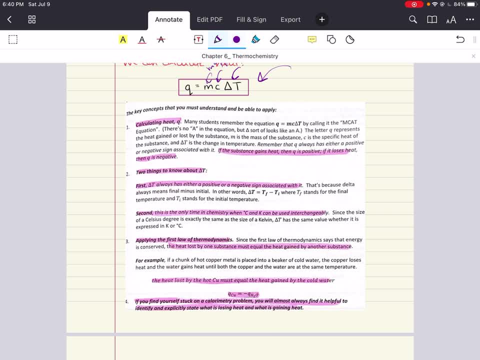 Must be equal to the heat gained by another substance. So if you're comparing, All right, If you're comparing heat lost by something, and it's equal. If you're, if you're calculating, All right, Heat lost by something versus heat gained by something, All right, You. 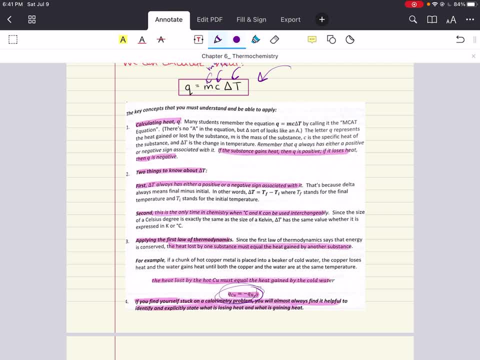 can equate it Right Because energy is conserved. So, for example, if a chunk of hot copper metal is placed into a beaker of cold water, the copper loses heat. All right, It loses heat and the water gains that heat because the copper is in the water. 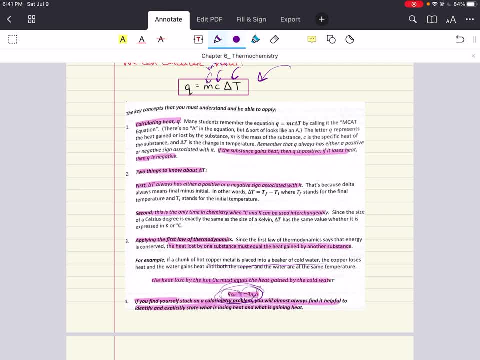 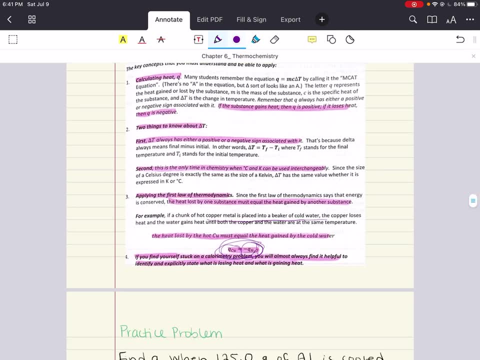 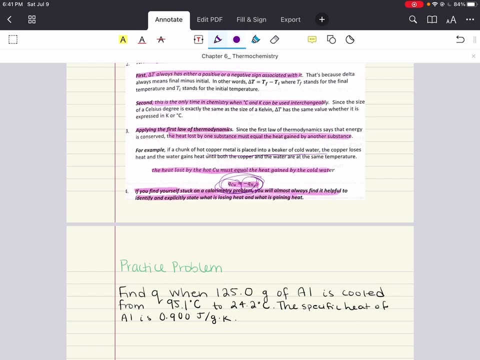 All right. So the heat lost by the copper is going to have to be equal to the heat gained by cold water, because of the first law of thermodynamics, because energy is conserved. So, keeping all that in mind, All right, Let's do a practice problem. Find Q when 125 grams of aluminum is cooled from. 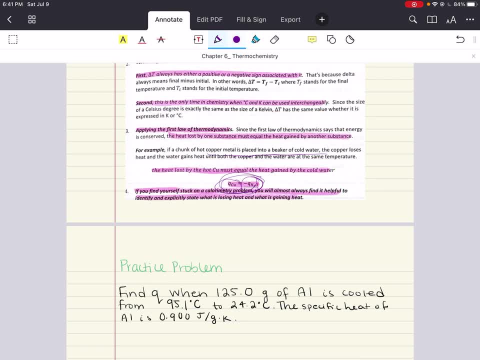 95.1 degrees Celsius to 25.1 degrees Celsius, All right. So if you're comparing heat lost by a copper, 24.2 degrees Celsius. And remember the specific heat of aluminum is 0.9 joules per gram times. 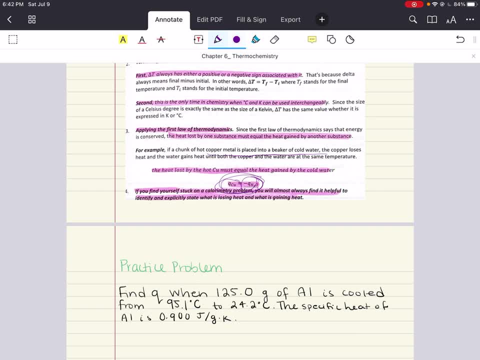 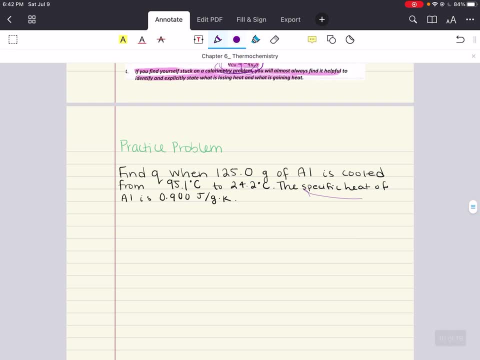 Kelvin. All right, Fantastic. Usually you will always be told the specific heat. You don't have to memorize a whole chart of specific heats. All right, Let's write first and foremost our formula. All right, Heat is equal to mass times, the specific heat times, delta T. All right, We're given our two. 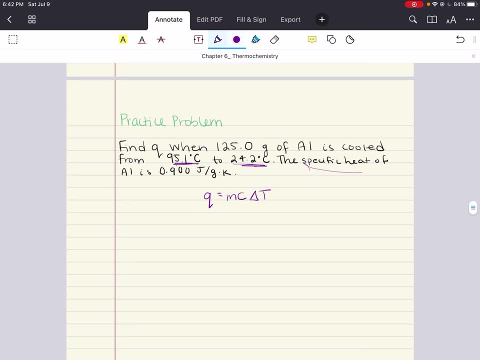 values. So we're going to start from and ending in. So what we can do is we can calculate delta T. We're going from 24.2 degrees Celsius. We're going from- sorry, 95.1 degrees Celsius to 24.2 degrees. 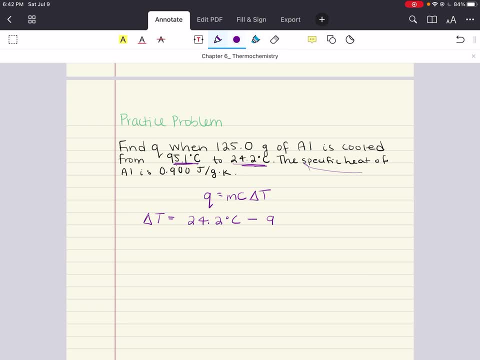 Celsius Delta, T delta- anything means final minus initial. So 24.2 degrees Celsius minus 95.1 degrees Celsius. All right, That's our temperature change. So we're going to start from and ending in. So what we're going to do is we're going to plug in our heat and we're going to plug in our heat. That's what.